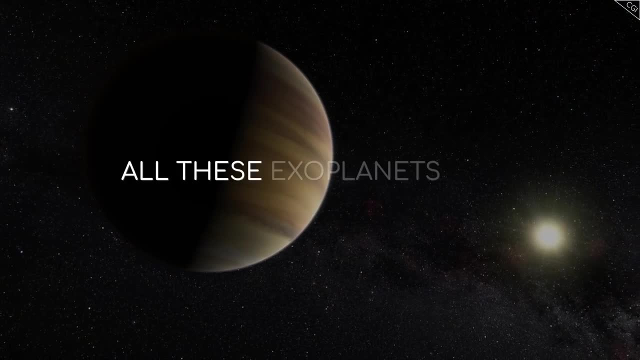 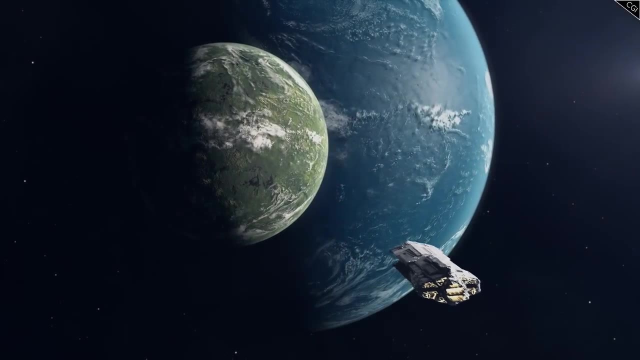 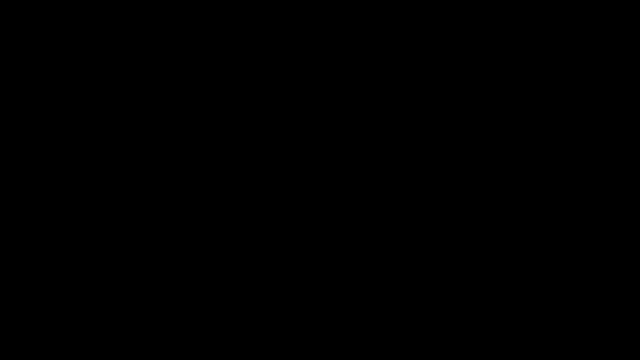 believe the hype. All the planets we've found so far have, to put it scientifically, sucked, And once you hear what I'm about to tell you, you'll agree that moving to any of them will be the last thing any sane person would want to do. 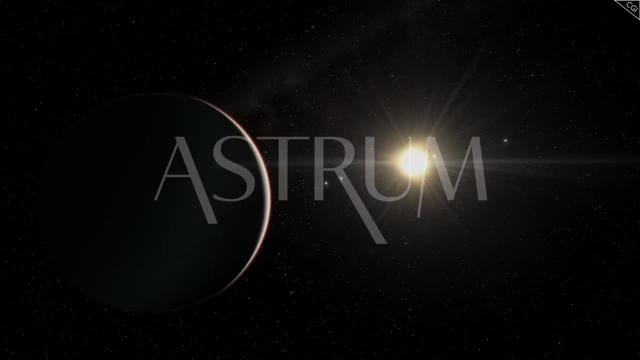 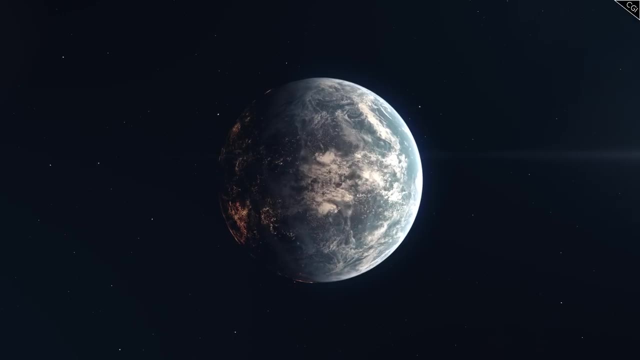 I'm Alex McColgan and you're watching Astrum. Join with me today as I give you the grand real estate tour on the potential Earth 2.0s we've discovered so far and explain why right now is the real question. 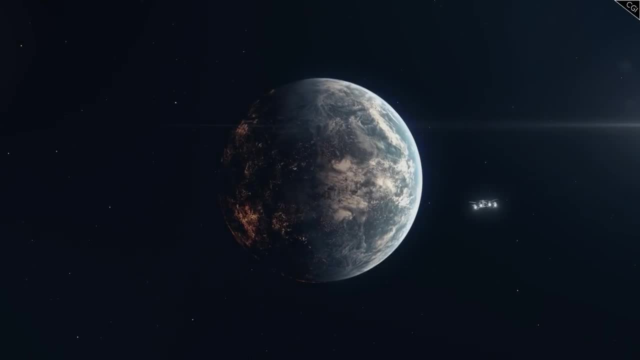 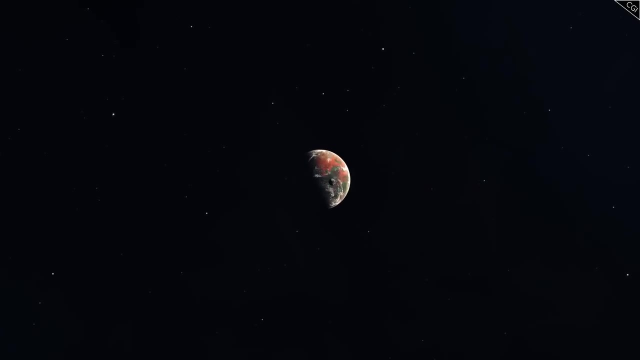 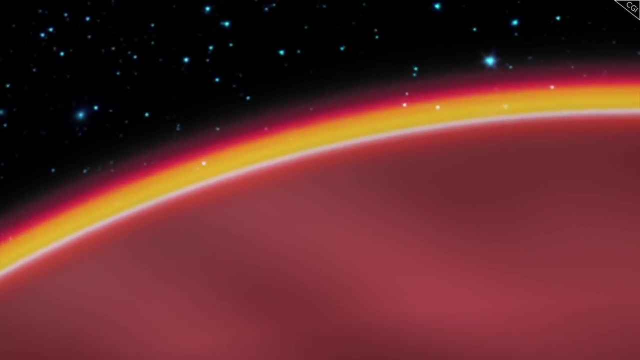 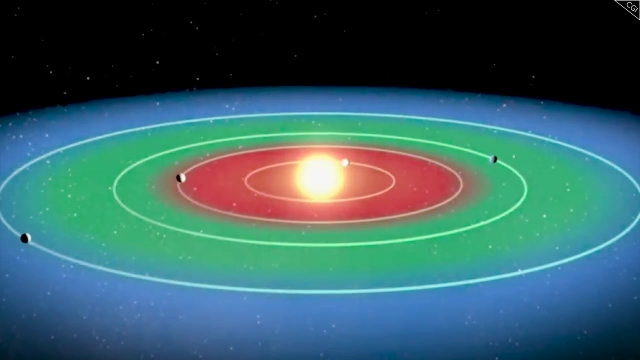 When choosing an Earth 2.0, just like with building a house- it's a good idea to start by establishing your non-negotiables. Some of this is fairly simple to consider, For instance, temperature. You want a nice temperate climate somewhere that's not too warm, and 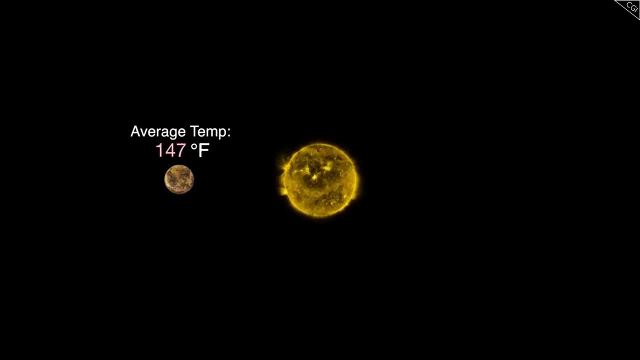 not too cold. Given that temperature drops the further you are from the sun, you want a temperature that's not too warm and not too cold. You want a temperature that's not too hot and not too cold. Every planetary system has a sweet spot where the temperature 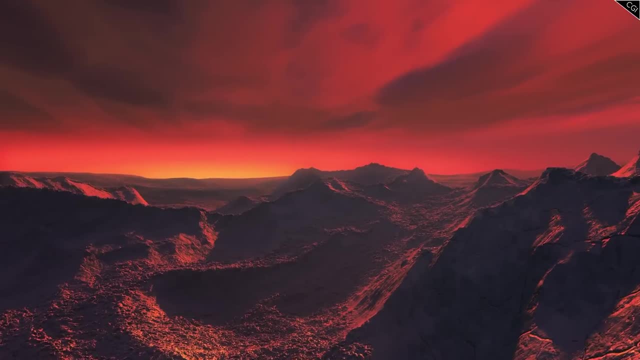 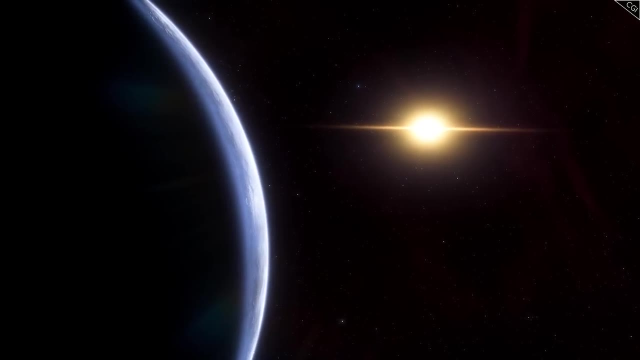 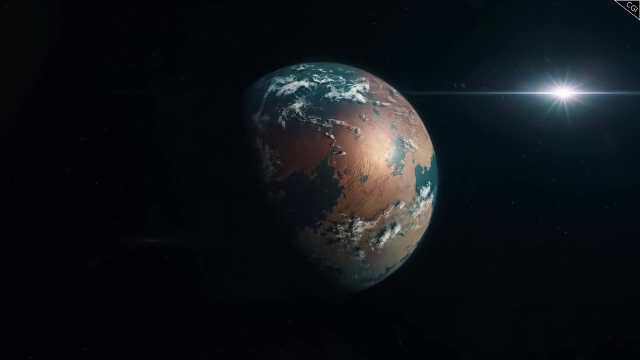 of a planet is likely just right: Not too hot and not too cold, Similar to Goldilocks and her bowls of stolen porridge. As a rough rule of thumb, if a planet is at the right distance from a star, it may well have a suitable temperature for us to set up shop. Of course, 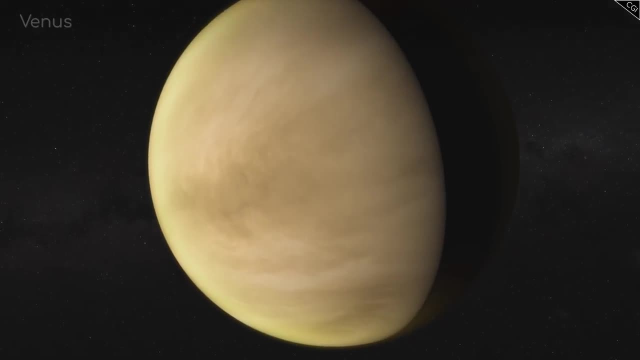 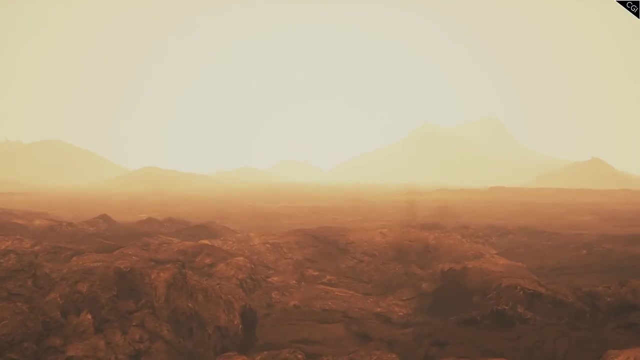 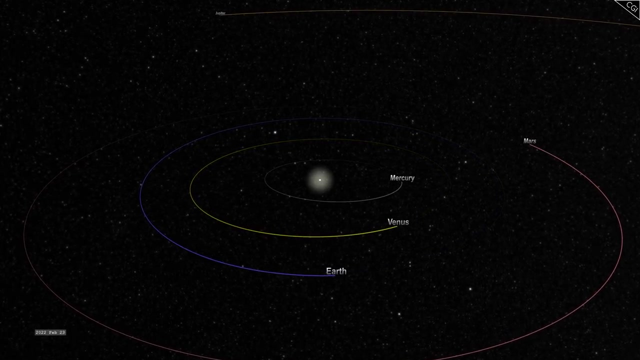 this is in no way a guarantee. After all, Venus, a planet residing in this zone, is in theory perfect, But its choking atmosphere makes it the hottest planet in our solar system, in spite of its relative distance from the sun compared with Mercury. So it's clear. 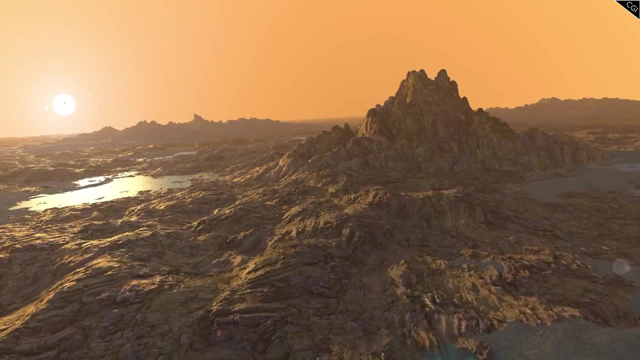 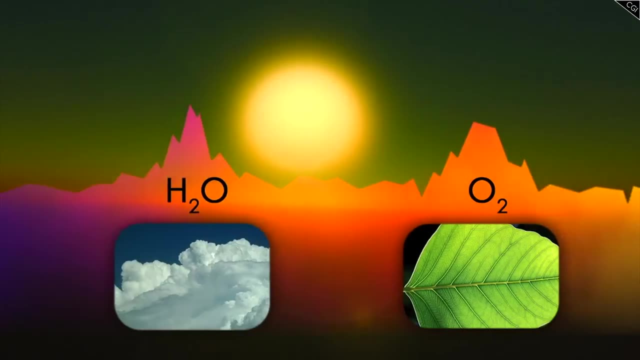 atmosphere also plays a part in all this. Speaking of atmosphere, that's also something you'll want to look for on Earth 2.0. Ideally something with oxygen and water vapour and without anything that would poison us, but at least something that could trap us. 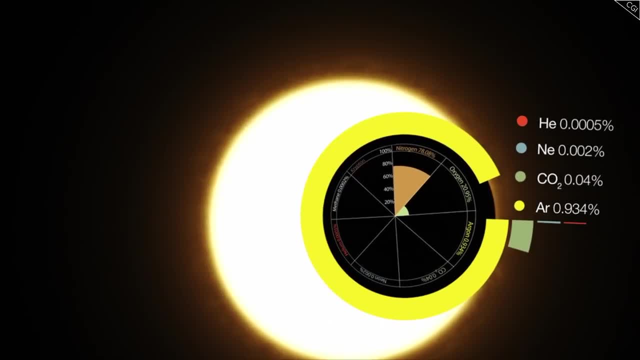 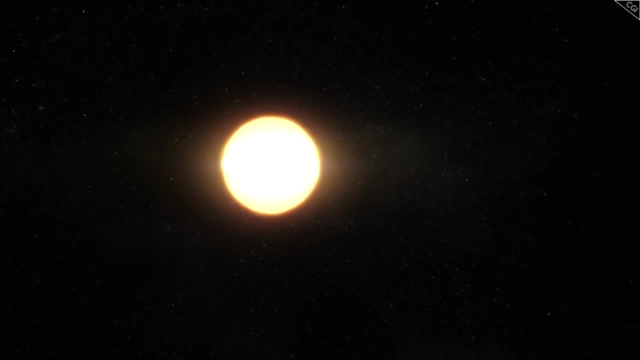 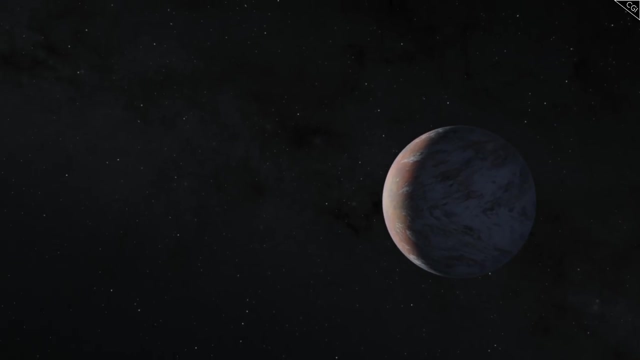 The Sun is also a very important planet and it is one of the most important planets in the universe. However, sometimes a non-negotiable is simply the neighbours that live close by. So let's consider the first major reason why most of the galaxy's exoplanets fall. 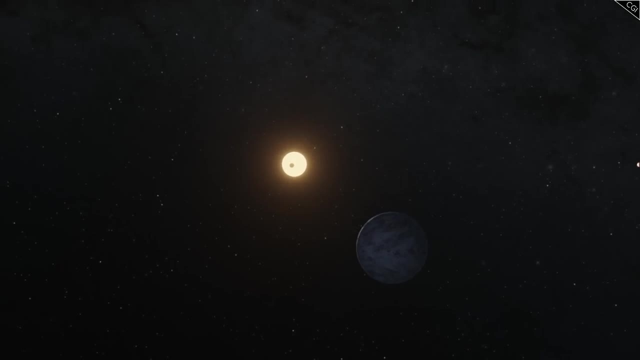 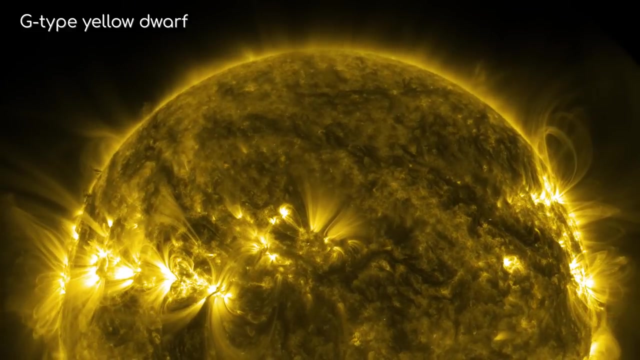 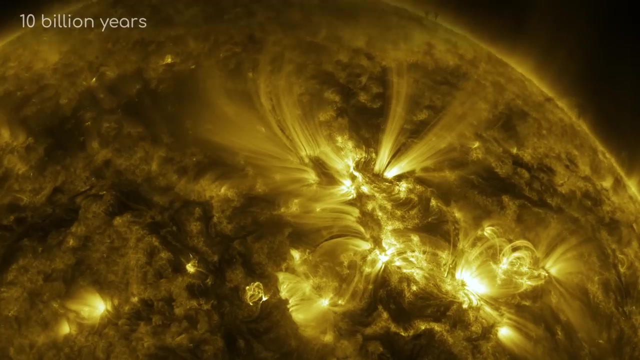 short, their neighbouring stars. Our own star is known as a G-type yellow dwarf, a relatively fast-burning, short-lived sort of star, at least compared to some of the other options out there. Stars like our Sun tend to live for 10 billion years before their cores collapse and they transform into a red. 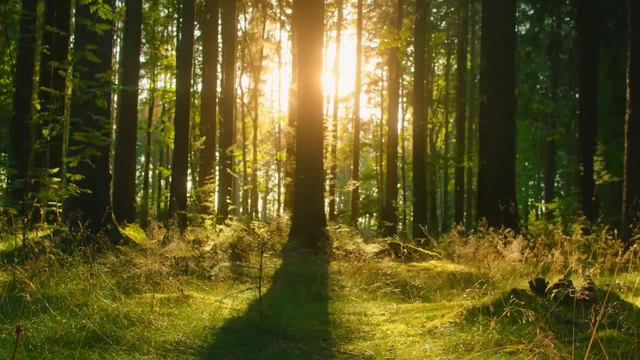 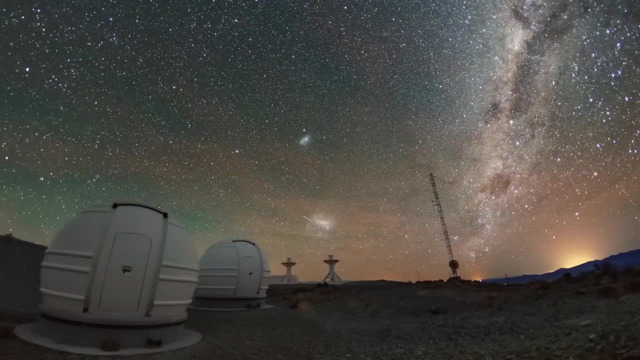 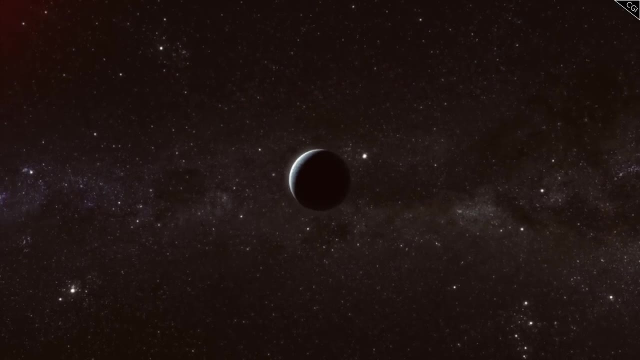 giant. It is stable, and that stability has been useful for the life that eventually flourished here. However, yellow dwarfs are far from common in the Milky Way. They represent only 10% of the total stars. Far more common in occurrence are the long-lived red dwarfs. 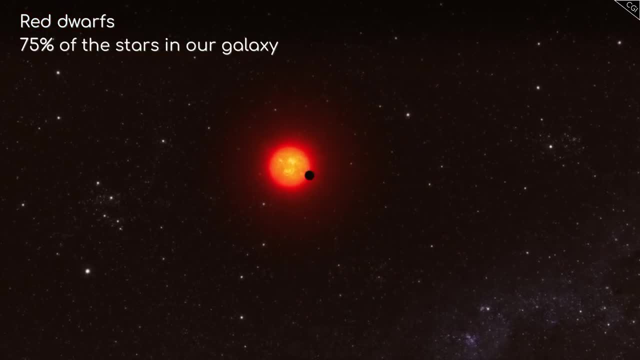 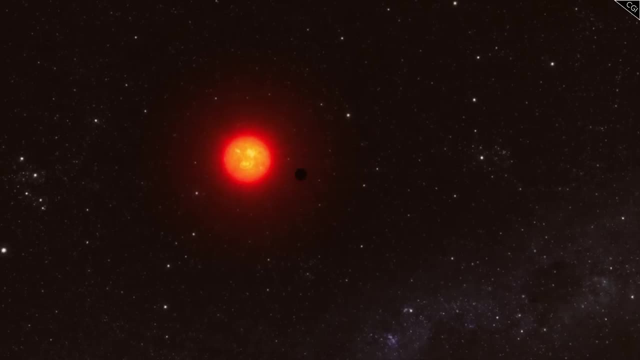 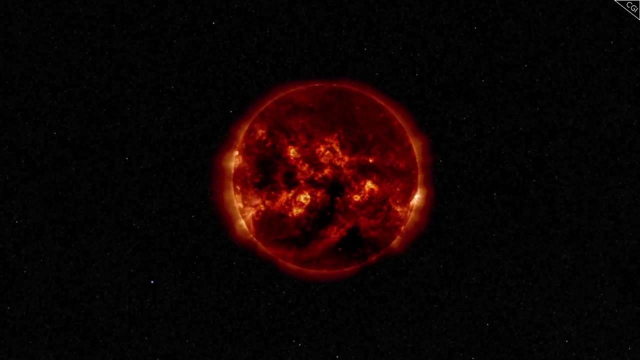 They make up 75% of the stars in our galaxy and can live for around 14 trillion years – longer than our universe has existed- which means we've never seen one die, so to speak. And unfortunately for the planets orbiting them, red dwarfs come with numerous. 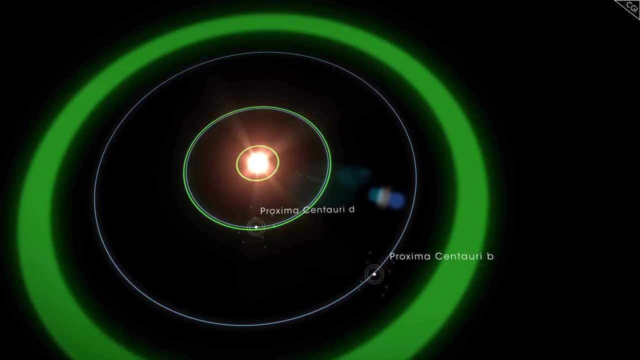 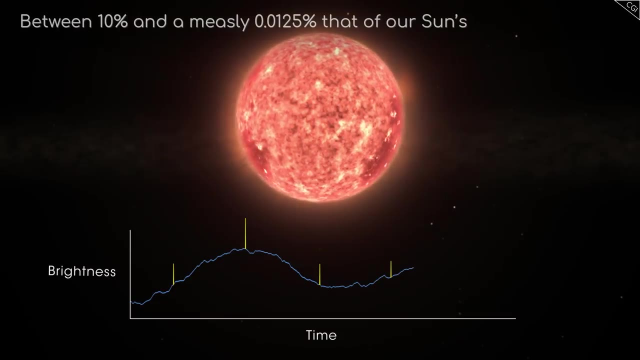 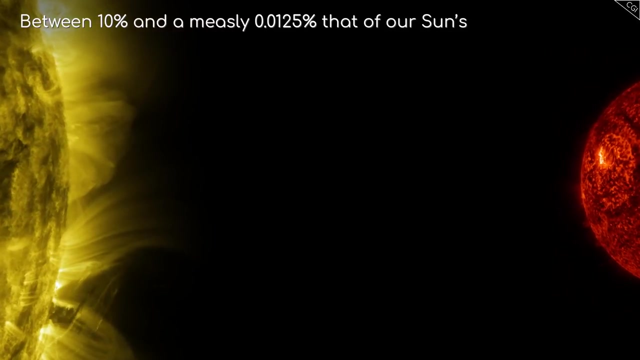 drawbacks. For starters, red dwarfs have a much closer Goldilocks zone compared to their yellow cousins. They burn less brightly. Unosity is between 10% and a measly 0.0125% that of our Suns. so unless you want to live, 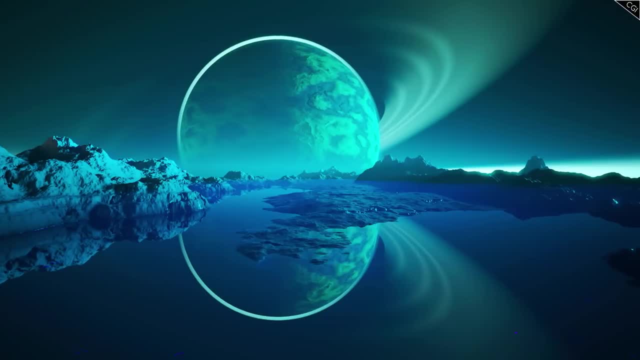 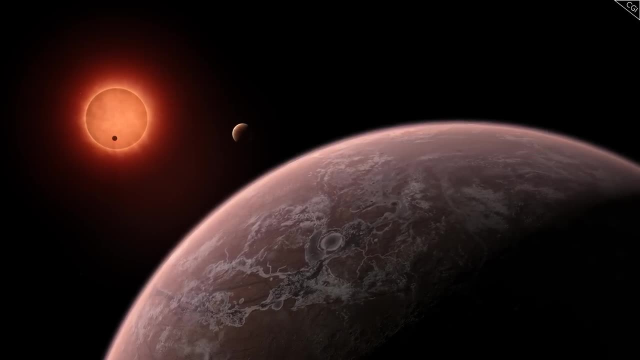 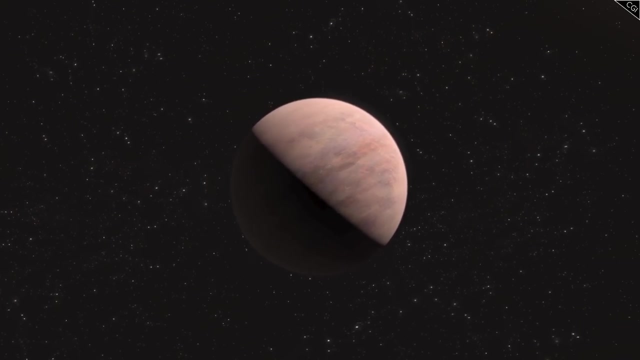 on a world shrouded in perpetual night – which sounds cold and depressing to me and will make growing plants a bit of a challenge – you'd want an Earth 2.0 to be a lot nearer to its red dwarf to compensate. This wouldn't be in and of itself a problem if it weren't. 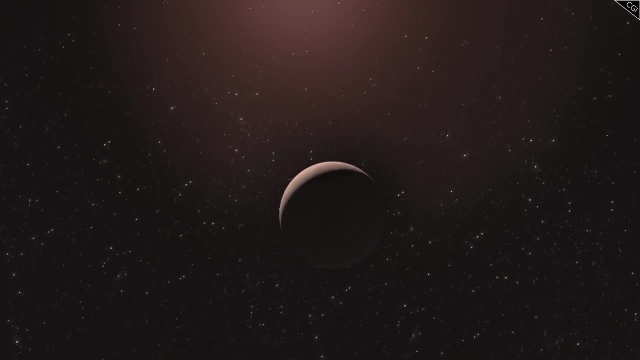 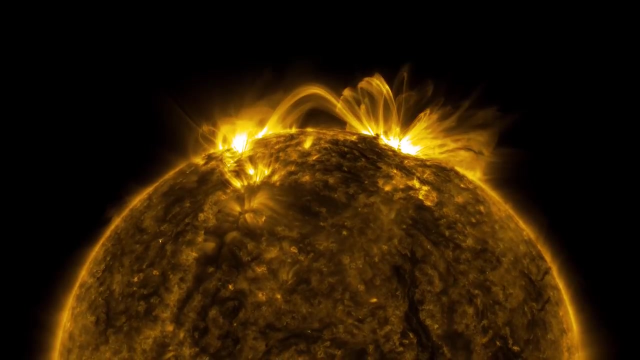 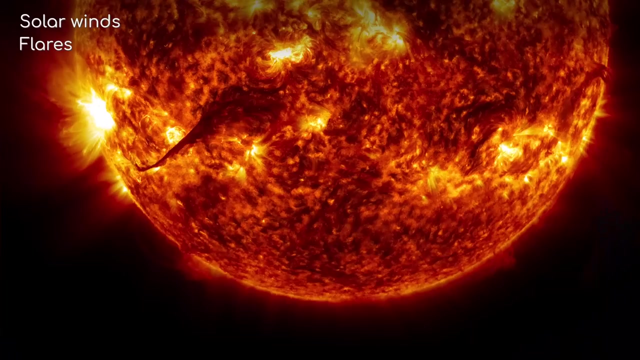 for the second characteristic of red dwarfs. Red dwarfs have a great amount of energy that is produced by red dwarfs. that makes them very unpleasant neighbours Their instability. Our Sun is the main source of our space weather – it shoots out a frequent stream of solar 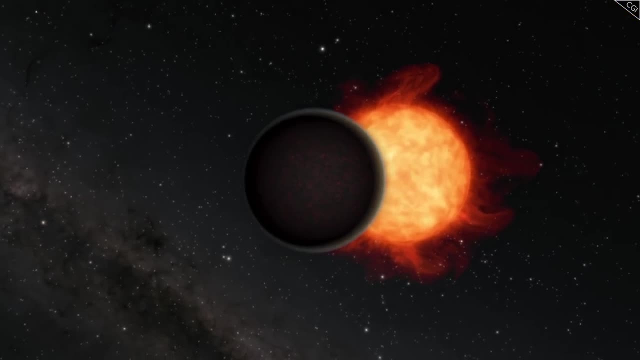 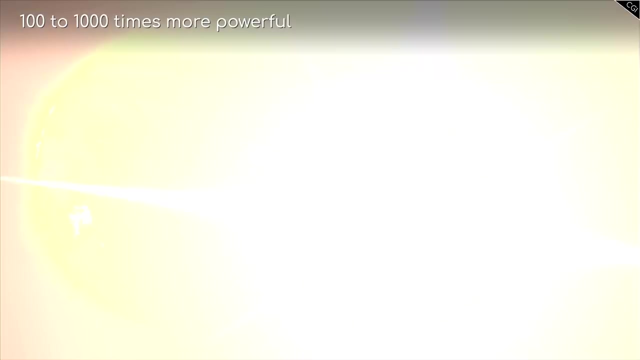 winds, flares and coronal mass ejections. However, this doesn't compare to the amount of space weather created by red dwarfs. Flares from red dwarfs can be 100 to 1000 times more powerful than those emitted by our Sun, But these red dwarfs' energy cannot beосpecified by the amount of space weather. 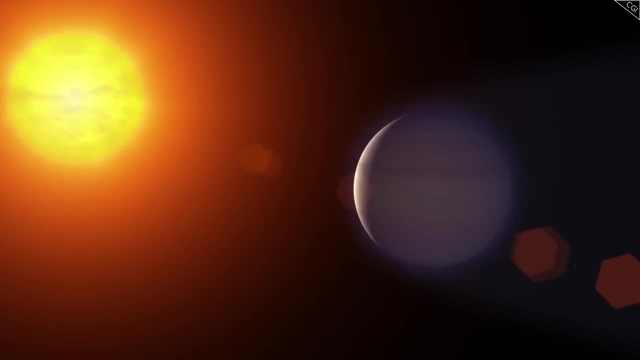 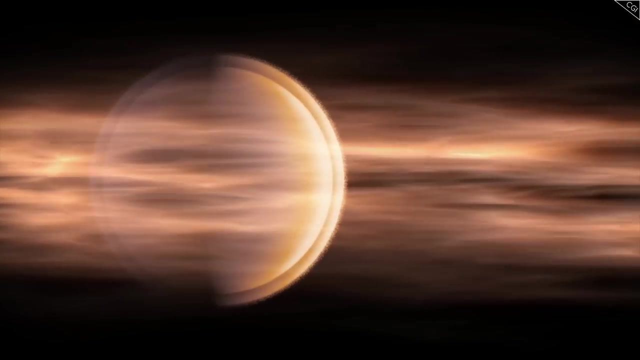 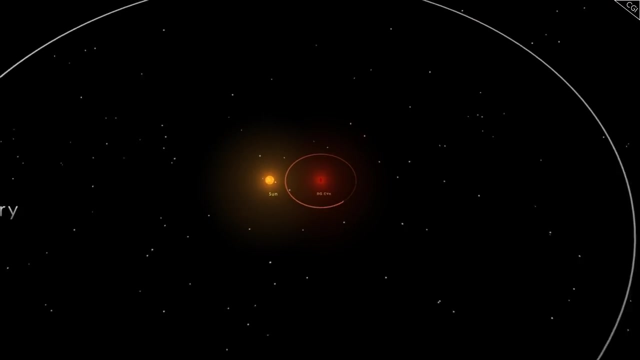 emitted by our Sun. The frequent bursts of plasma and radiation coming from red dwarfs are powerful and dangerous enough to strip away the atmosphere and even boil liquid water on planets in the habitable zone. And, given how much closer planets are to their star in a red dwarf system, the odds of life getting enough time to arise before being hit with? 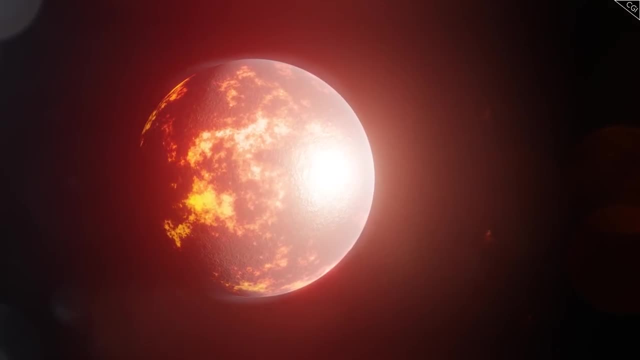 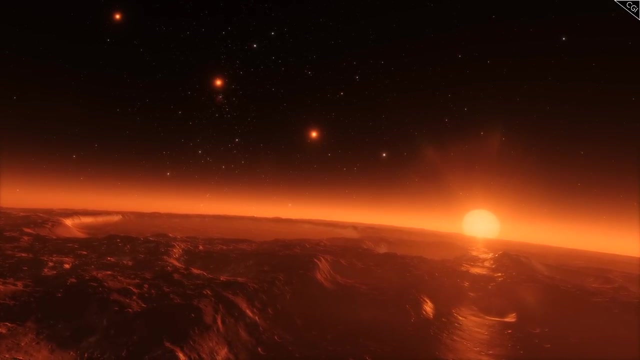 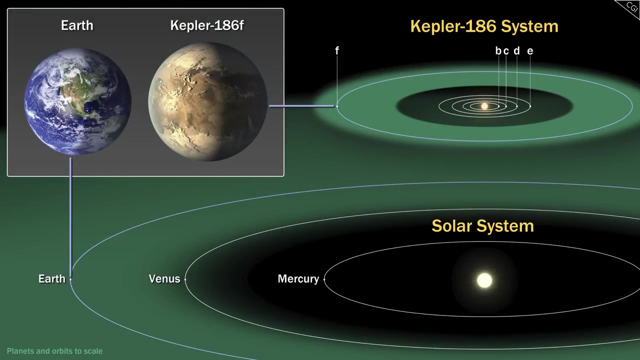 a life-sanitising dose of X-rays is pretty slim. If you want to live on a planet around a red dwarf, you'll likely need some serious sun cream. This rules out many known exoplanets, such as astronomer favourite Kepler-186f, which. 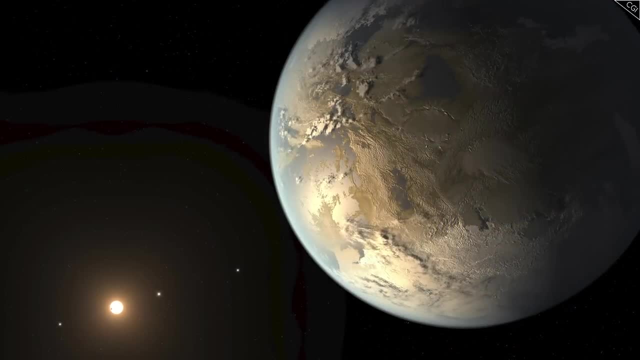 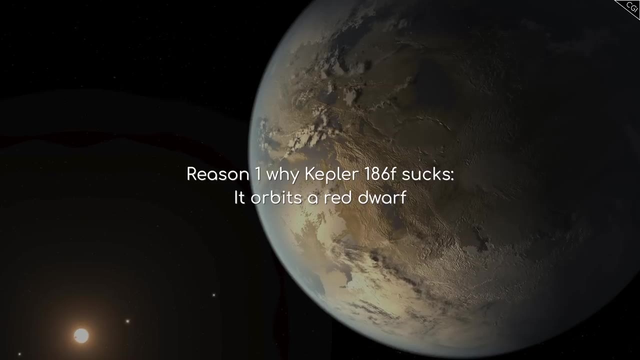 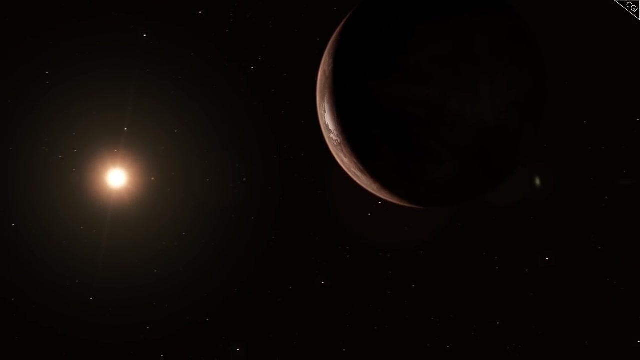 some scientists hoped might be habitable. While it may be possible to live for a time in quite uncomfortable conditions in a deep underground bunker on such a planet, the experience would hardly be pleasant. But even during periods between harsh solar weather events, there's another problem. 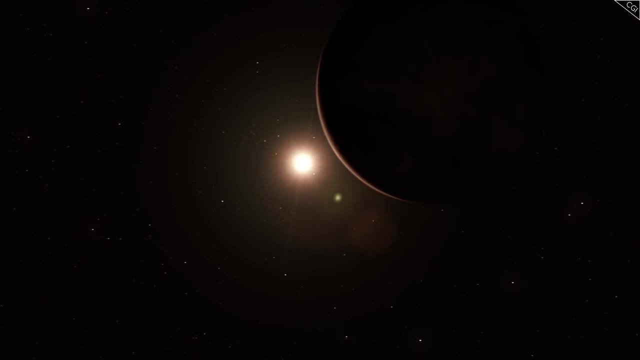 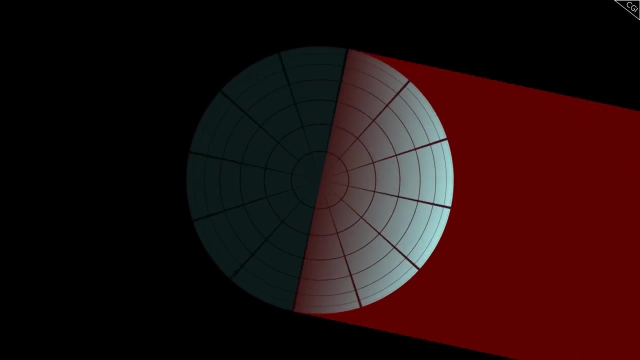 with planets around red dwarfs – their tendency to be tidally locked. Being tidally locked means that the same side of the planet always faces the star as it orbits. There is no rotation between day and night. One side of the planet is in perpetual. 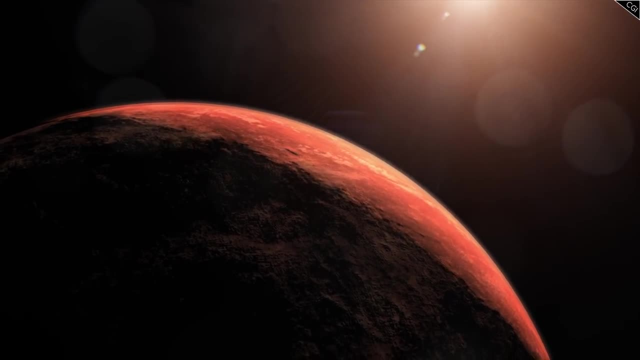 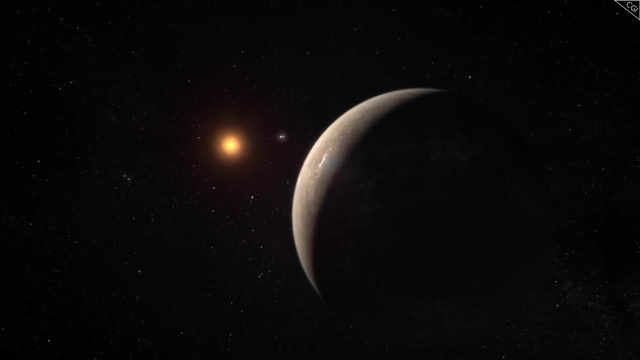 heat and the other side in permanent shadow. Due to gravitation, the planet is always in constant heat and the other side in permanent shadow. Due to gravitational constraints, planets near their sun have a tendency towards being tidally locked. Just take a look at Mercury, with its day that lasts 176 Earth days or 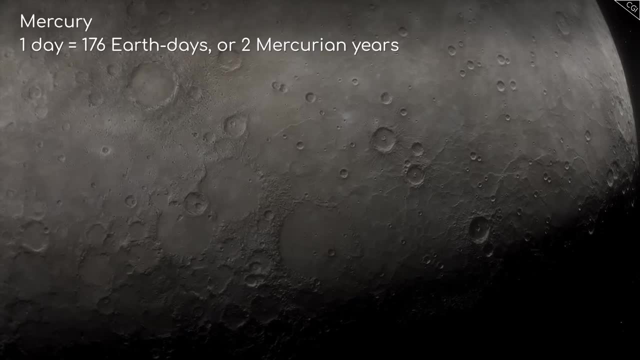 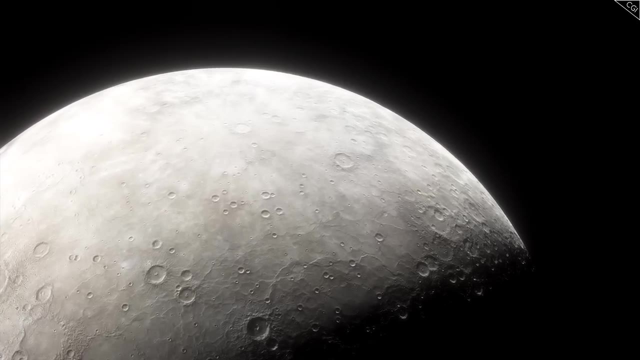 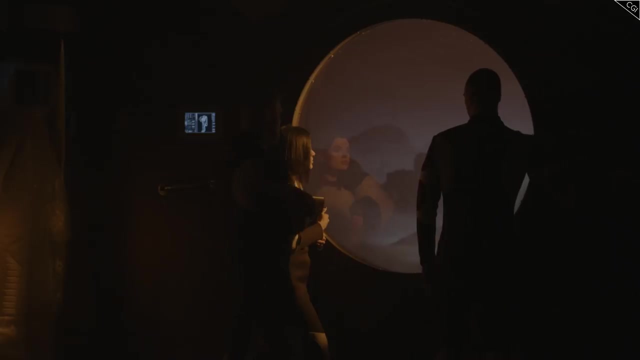 two Mercurian years. This lack of rotation could render most of the planet uninhabitable. You'd either face scorching desert-creating heat on the day side or freezing ice on the night side. Even if humans tried to live in the narrow band of twilight that would ring. 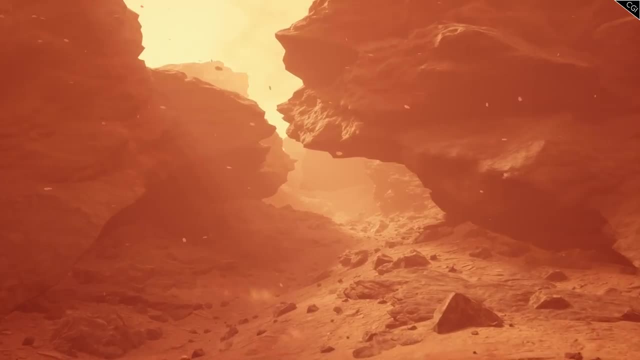 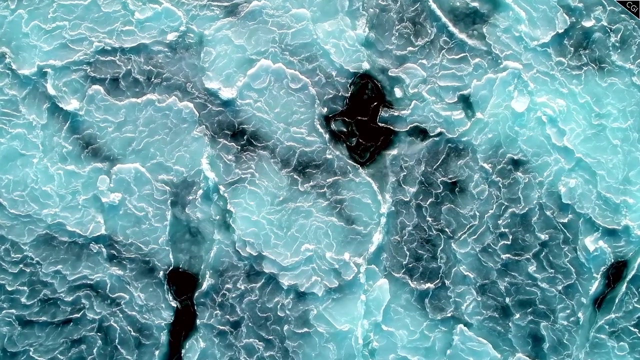 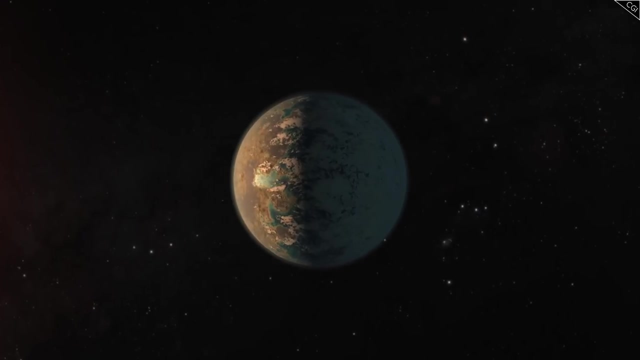 a tidally locked planet, liquid water might prove difficult to find. Any moisture in the air that found its way to the night side of the planet would get locked there, solidified as ice. Overall the planet would be very dry, and even in the twilight zone there. 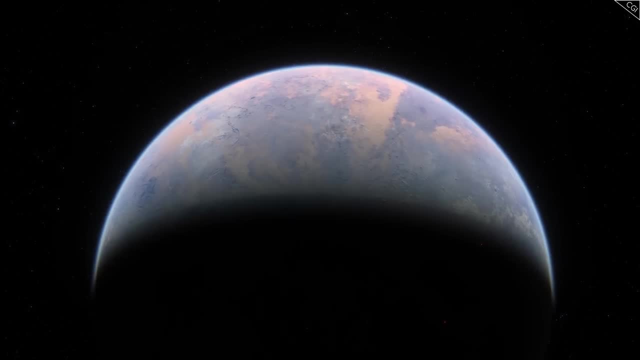 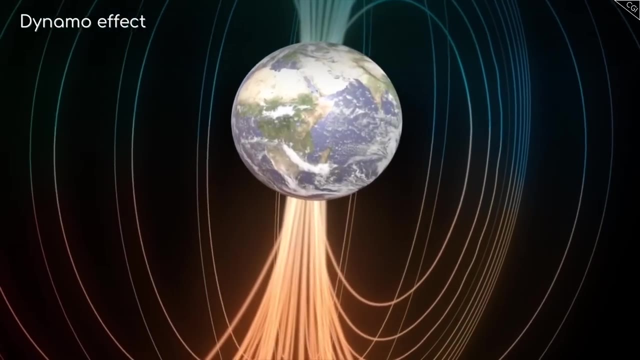 would be no rain, And that's not to mention the low power of a magnetic field that would likely be found on a tidally locked planet. The dynamo effect that powers the magnetic field on Earth is thought to be influenced by the Coriolis effect. the rotation of the 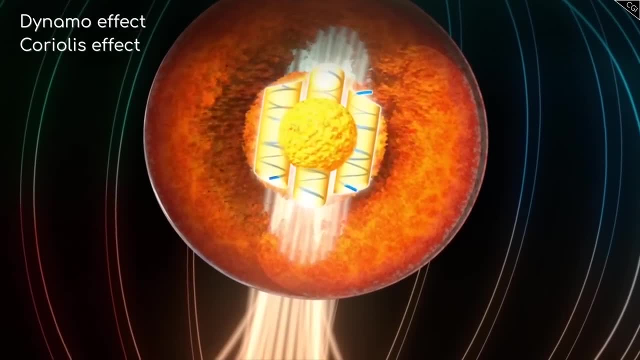 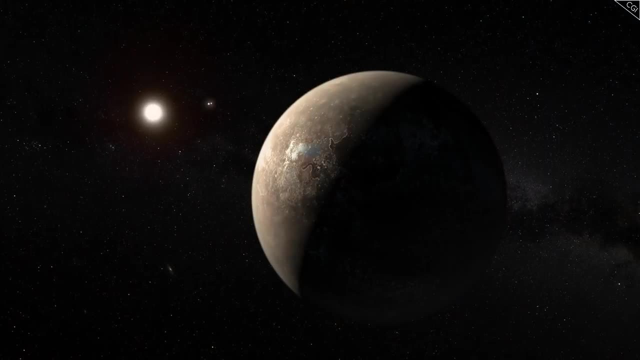 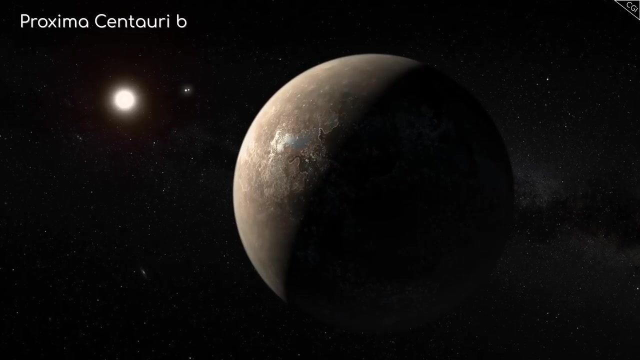 Earth imparting momentum to rising and falling liquid metal in its core. Without this rotation, such a magnetic field would be inevitably weaker. So I'm sorry to say that this rules out planets such as Proxima Centauri b, our closest exoplanet. 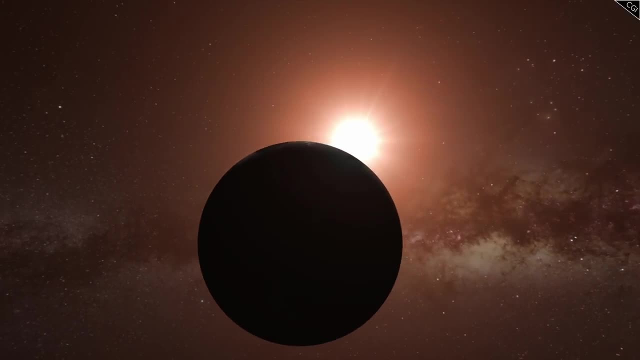 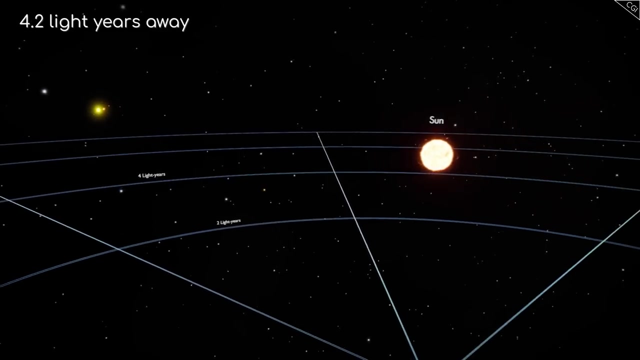 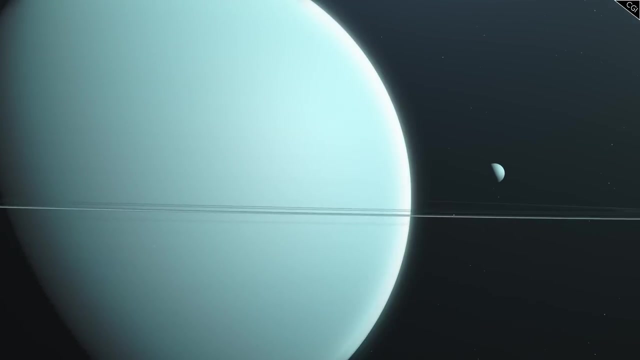 Proxima Centauri b is otherwise an interesting candidate. Its closeness makes it one of the easiest planets to get to for us. situated only 4.2 light years away, It's thought to be a rocky, Earth-like planet, which is convenient, as living on a gas giant would. 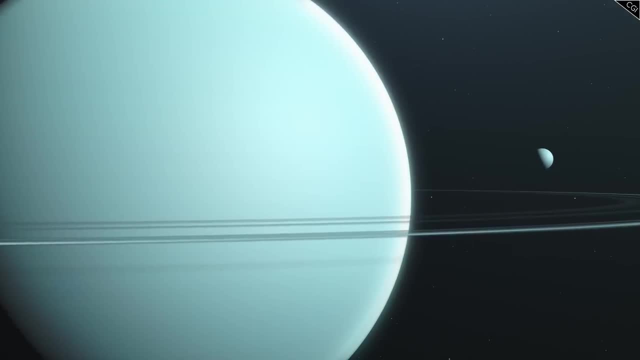 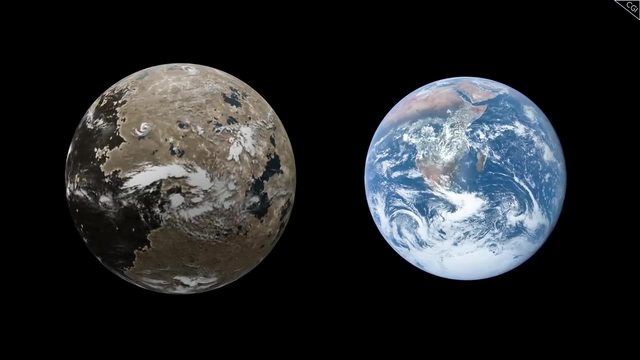 be challenging to anyone with a fondness for solid floors beneath their feet And most compelling. its mass and radius are very similar to Earth's, meaning it has a similar gravity. Why is this important? Let's compare it with another Earth-like planet. 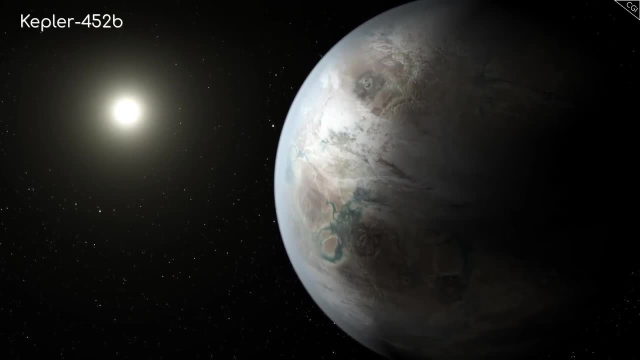 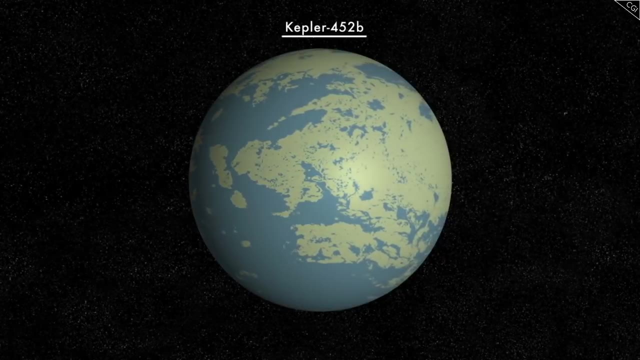 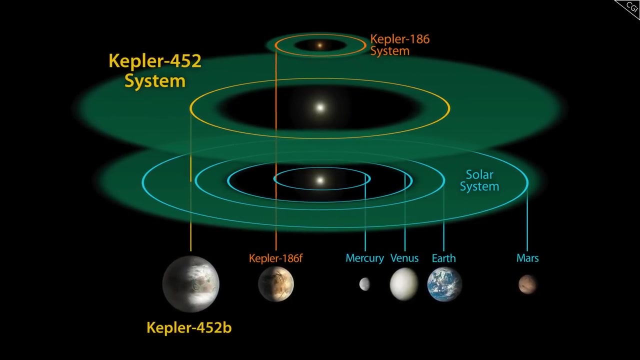 Earth 2.0 contender, Kepler-452b, The first planet to ever be referred to by that title, and the planet described by a NASA scientist as the closest twin to Earth. Kepler-452b has much to recommend it: It is orbiting around a yellow dwarf like us at a similar distance. This means 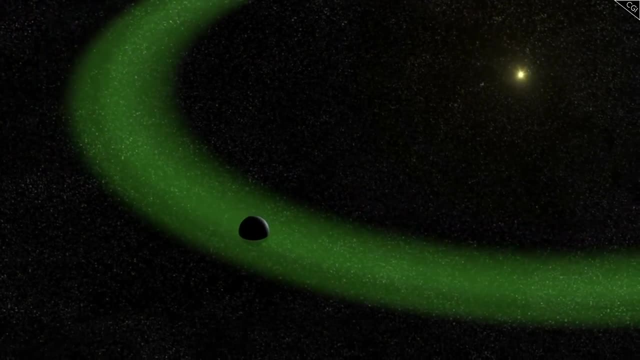 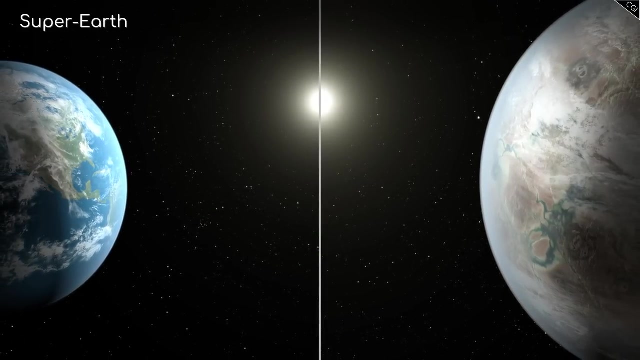 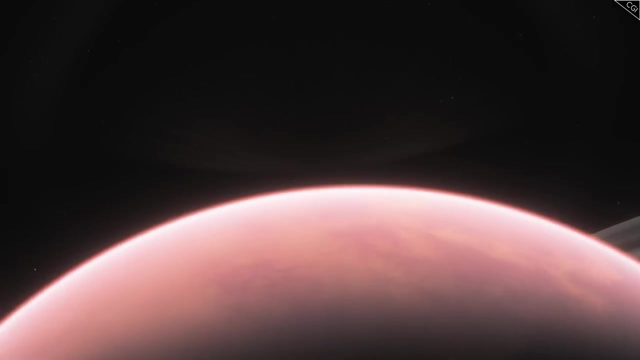 it's in the Goldilocks zone. that makes liquid water on the surface possible. However, it is a super-Earth. This means it has a mass and radius combination that makes it about twice that of Earth's. When it comes to gravity, how much is too much? 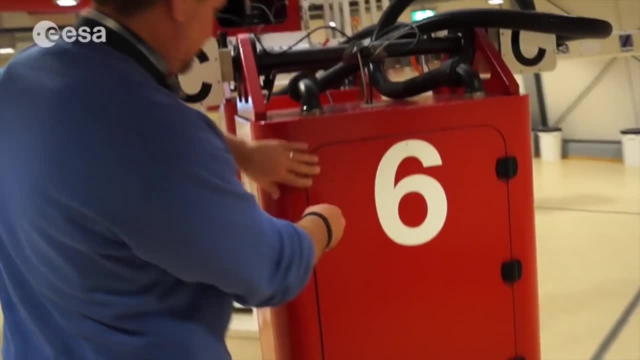 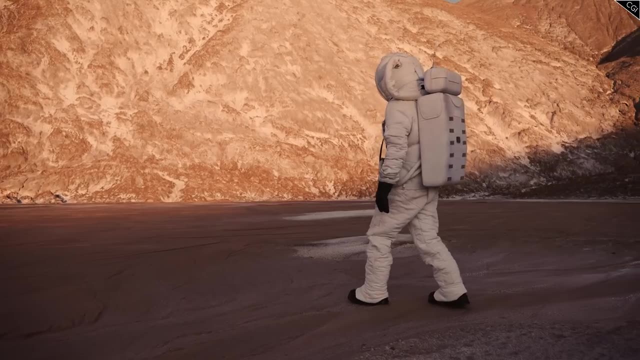 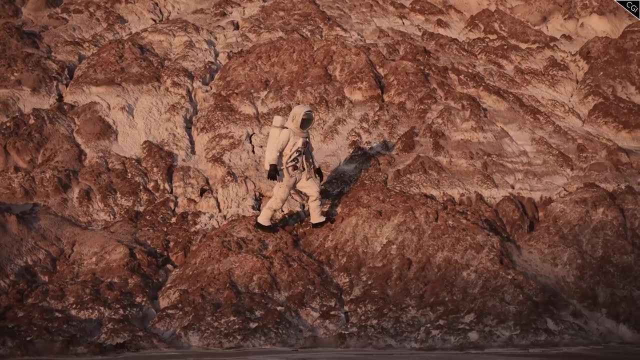 Some scientists researching the question put the figure at 4 times Earth's gravity, this being about the limit of what a human could survive. However, even living in just twice Earth's gravity could get rather uncomfortable To properly visualise this, or at least get a rough approximation of it. 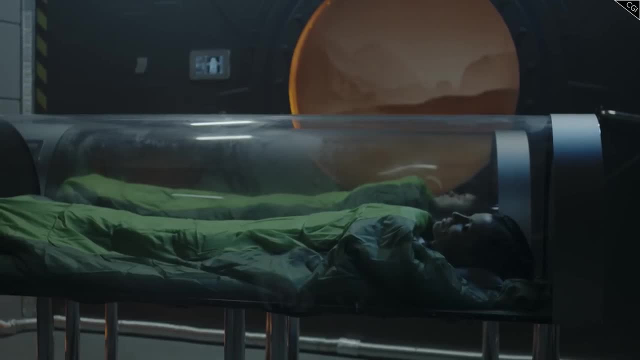 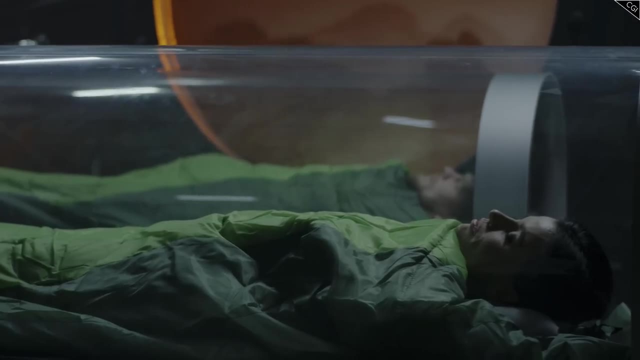 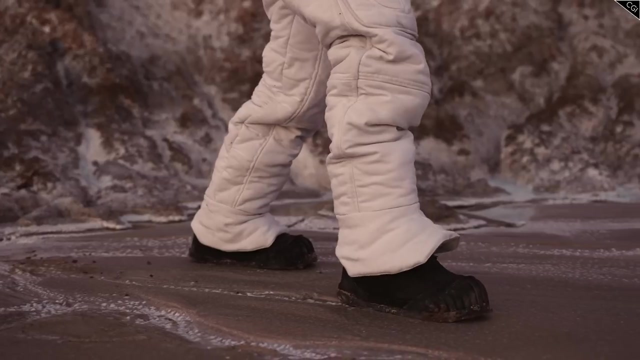 imagine lying down, but then imagine a second person lying on top of you, putting all their weight on you. This is your night, every night, every breath being fought for. Come daybreak, you must lift that extra person up, haul them onto your back and then carry them with you. 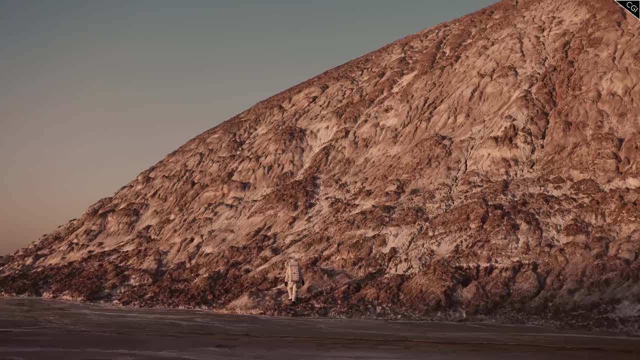 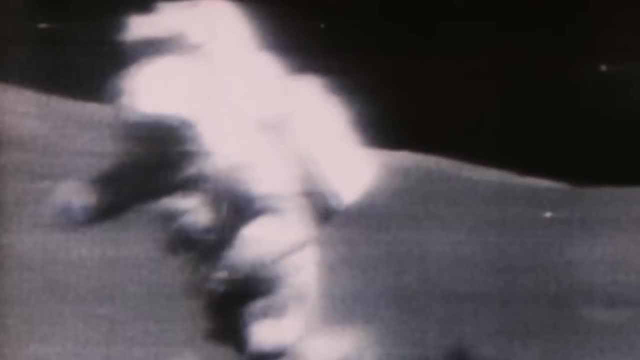 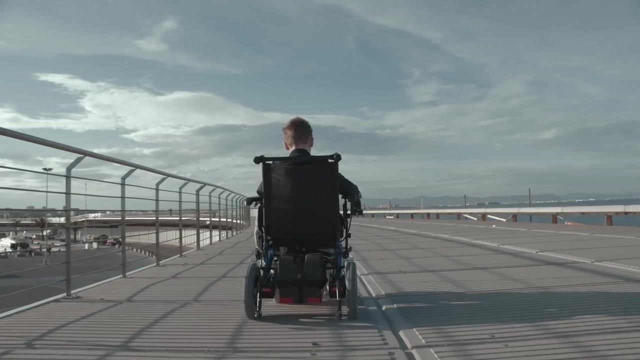 everywhere. you go Everywhere And be careful not to fall, as suddenly it's much easier to break a bone. Falling downstairs is no longer painful, it's likely lethal. Everyone must do this: the elderly, the infirm, small infants trying to take their first wobbling step. Keeping this in mind, 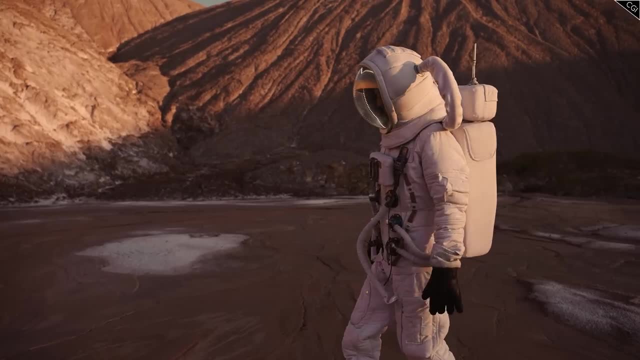 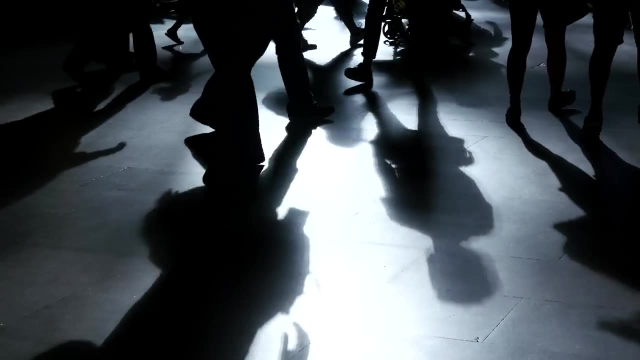 it's easy to grasp just how exhausting life in double gravity might end up being. If you're a bodybuilder or athlete, you will likely be alright, but for most people on Earth it would be a slow torture, Your heart furiously beating to move. 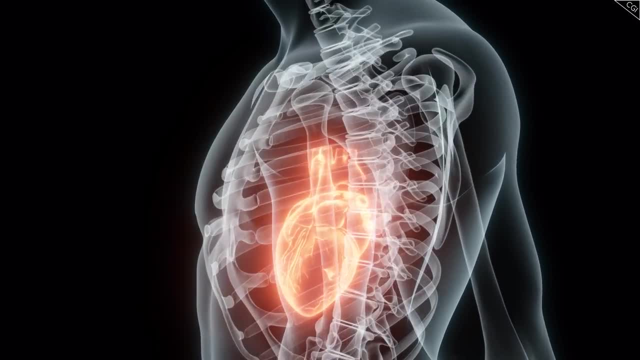 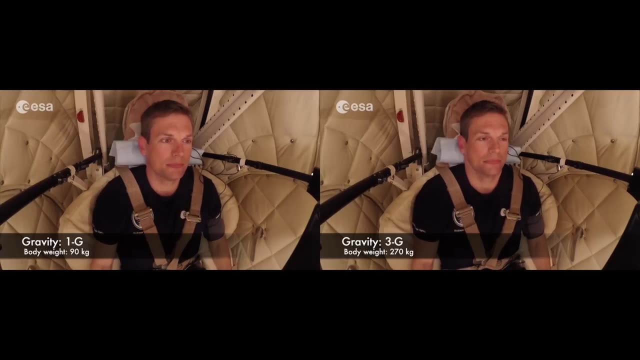 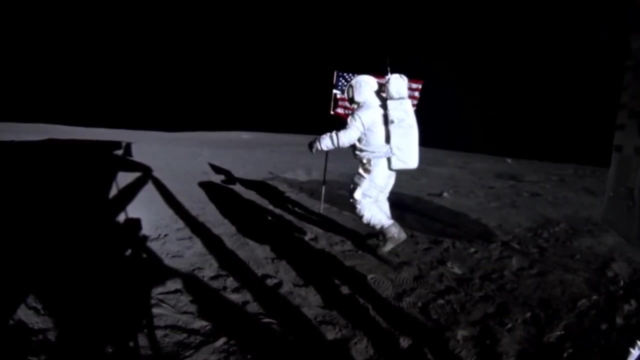 your blood around, making it feel like you're running even when you're standing still. And if you want to triple the gravity, add an additional person on top of that And things don't get much better. going the other way, Sure, everything is much easier as that weight is lifted. However, 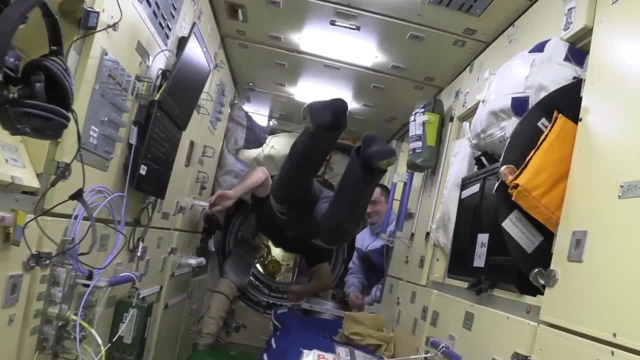 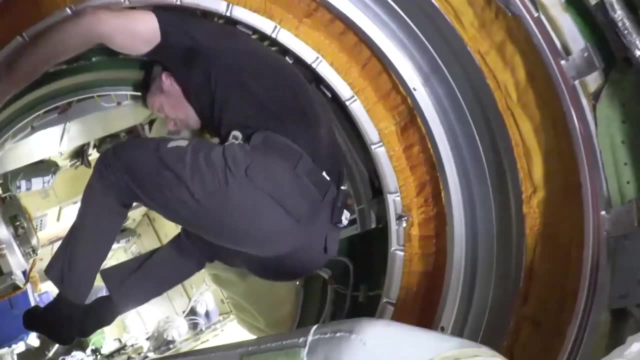 living under reduced gravity comes with a host of health risks that we can see from astronauts who've spent just a few months on the International Space Station. Over time, the calcium bleeds out of your bones, causing them to become brittle. Your muscles 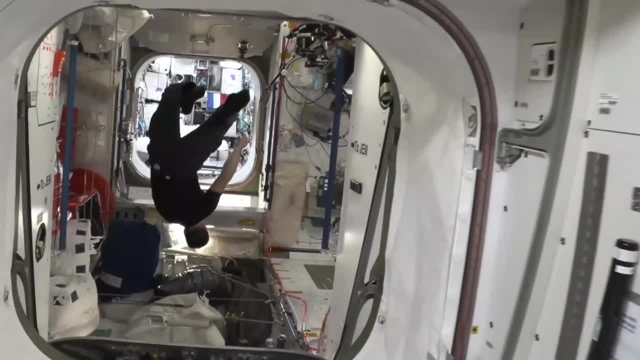 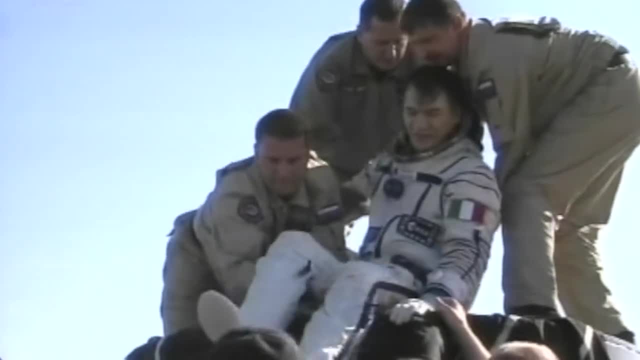 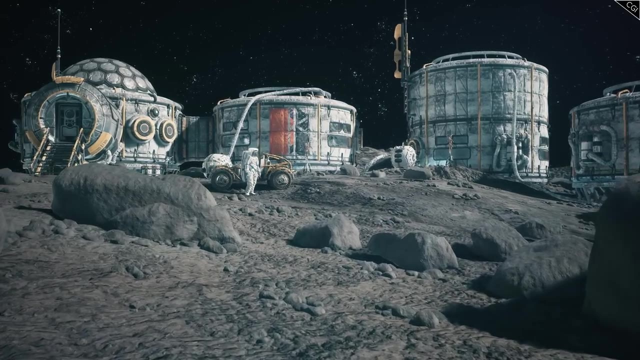 atrophy, Your heart develops issues, Your immune system suffers. All told, even if you're exercising every day, your long-term prospects aren't looking good in a low-gravity environment, a fact that is challenging NASA scientists as they try to figure out how to set up human outposts on. 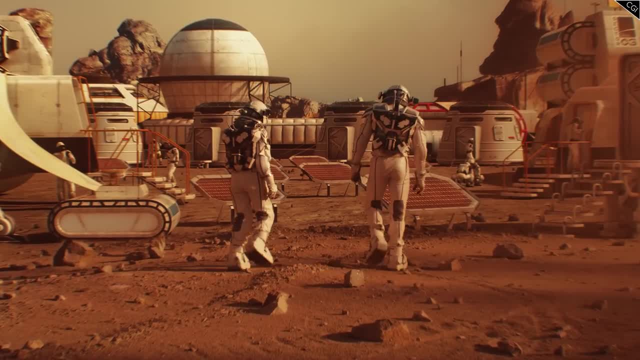 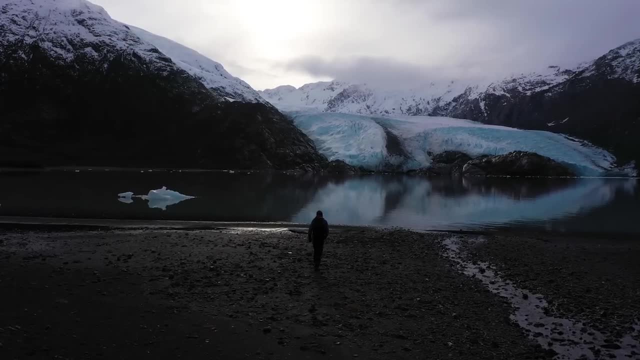 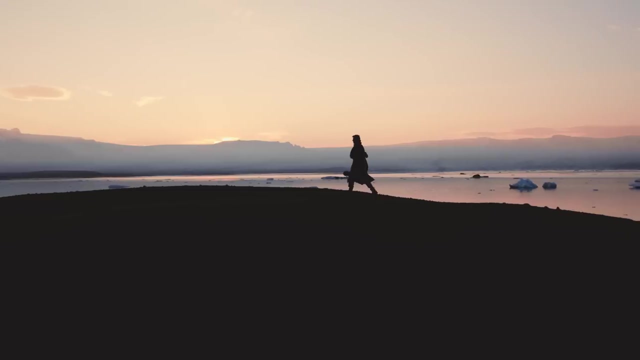 places like the Moon or Mars, where astronauts might go to live for just a few years. Humans have spent millions of years adapting to life on our planet. We're very used to how things are here. We're just not suited to anywhere else. We've not evolved to face such conditions. 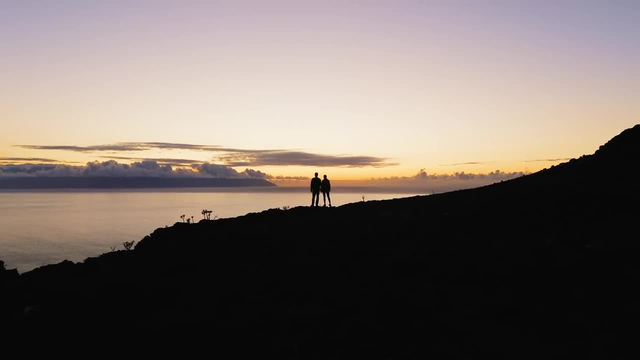 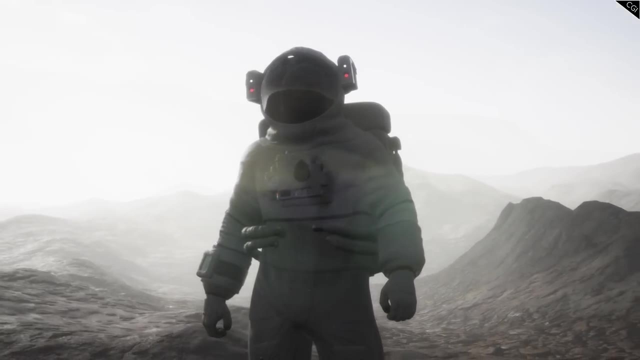 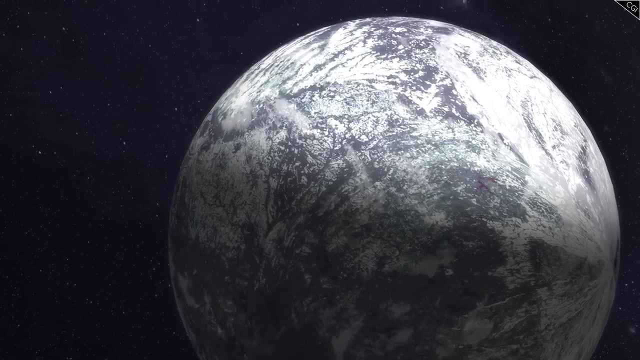 In some respects it's a testament to how well we've acclimatised to the environment we were born in, but it's a big obstacle, if ever we want to live anywhere else. The Hunt for Earth 2.0. And so the hunt for Earth 2.0 goes on. As I mentioned, there are likely billions of 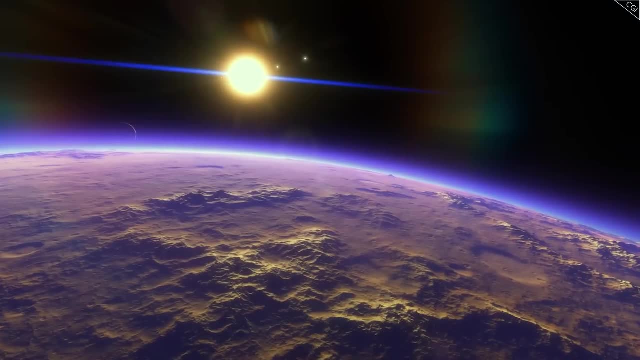 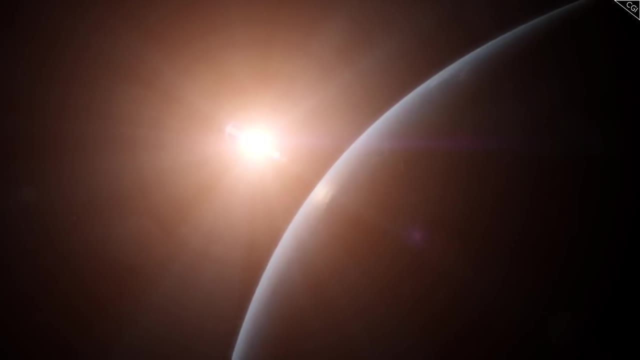 undiscovered planets in our Milky Way Galaxy. The odds of at least one being out there that meets our criteria for gravity, temperature, lack of life-threatening radiation and presence of atmosphere and water are high enough to be a certainty. The odds of one being out there that meets our criteria for gravity, temperature, lack of life-threatening radiation and presence of atmosphere and water are high enough to be a certainty. 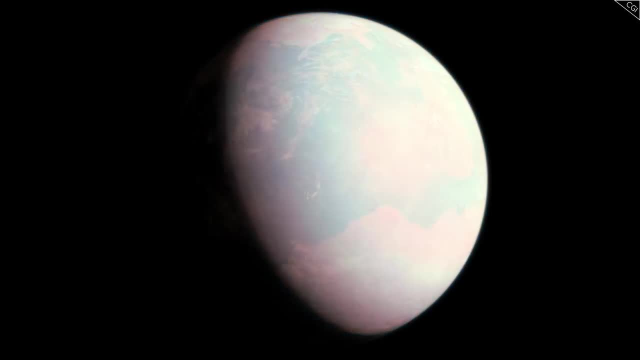 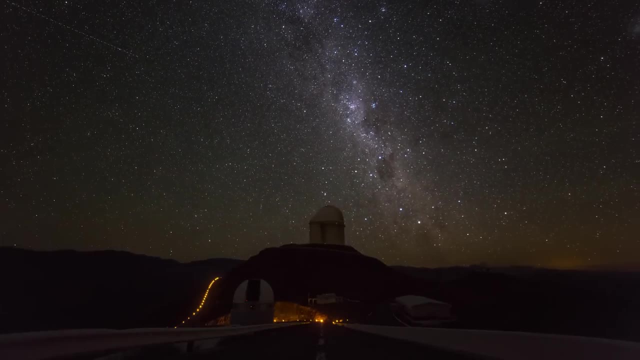 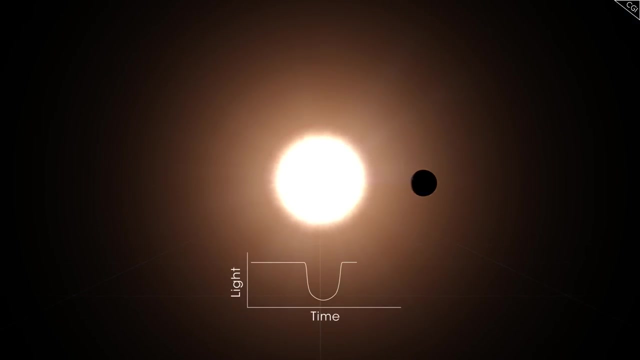 Actually finding one that meets the criteria is much more of a challenging task, particularly when most planets are still invisible to even our strongest telescopes, except for a brief moment when they pass in front of a convenient star and block out its light. If someone tells you that they've already found Earth 2.0, I'd take it with a pinch of salt. We 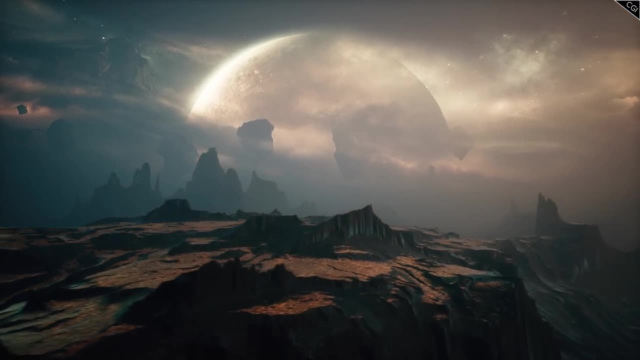 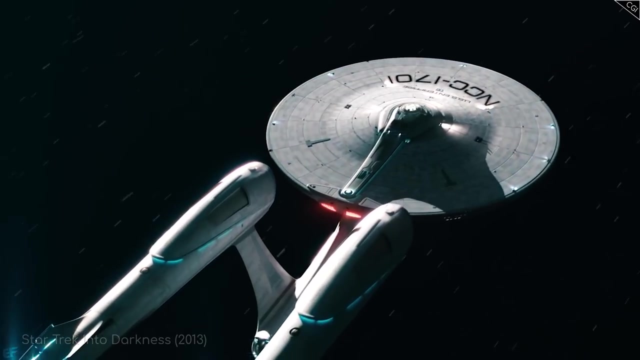 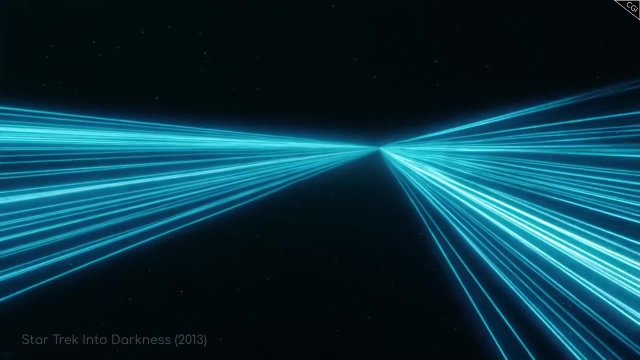 won't ever really know that the planet is actually suitable for human life until we somehow cross the gulf of space and go there to see it in person. Of course, until we discover how to do that, it's all a bit of a moot question anyway. 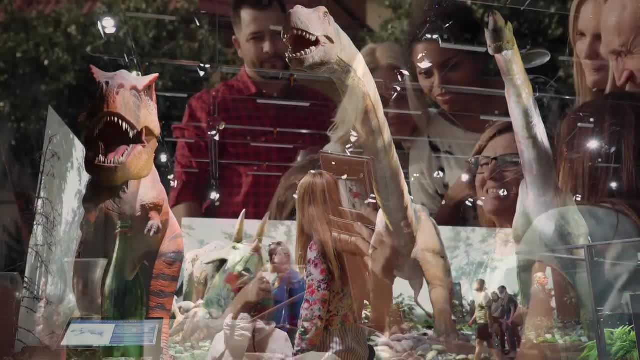 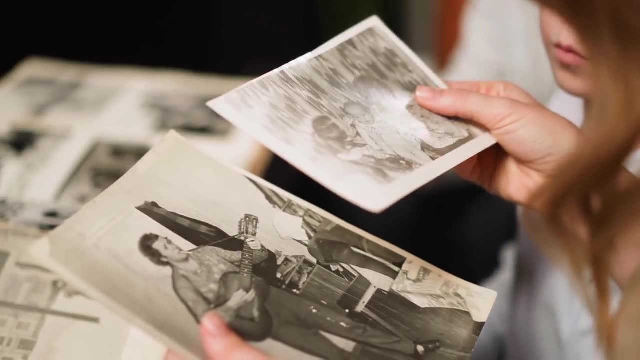 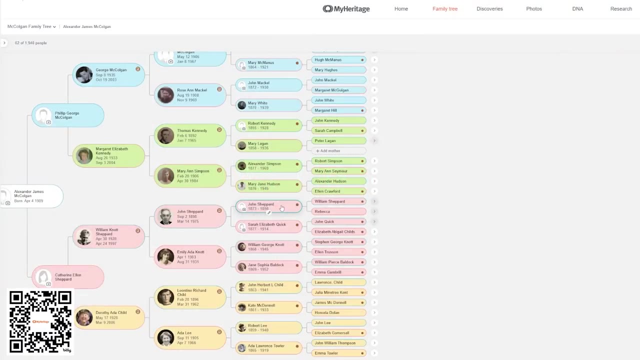 Life has developed on this Earth for millions of years, but we sometimes forget the personal connection we have to those who've gone on before. Have you ever wanted to know their stories? You can. thanks to my partner for today's video: MyHeritage. I have a Canadian great-great-grandfather who was 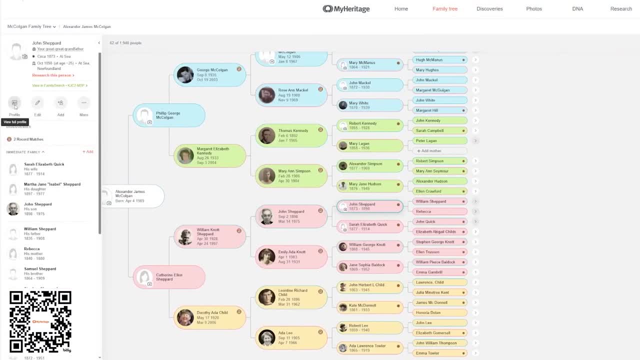 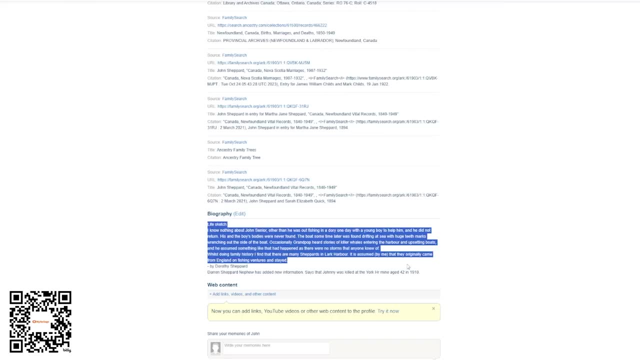 born at sea and died there. He and a boy went fishing one day and were never seen again, although the boat was later found with giant bite marks taken out of the side. I'd never heard this story before, but I found it as I started to delve into my family history. 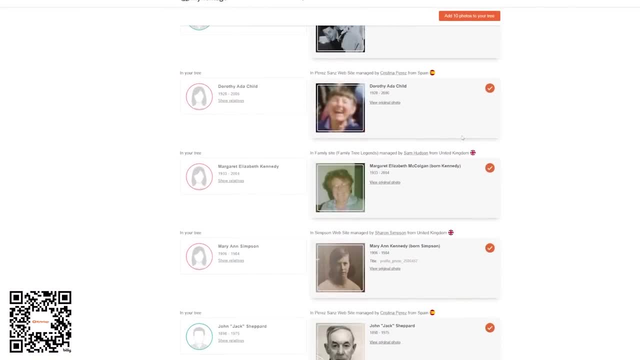 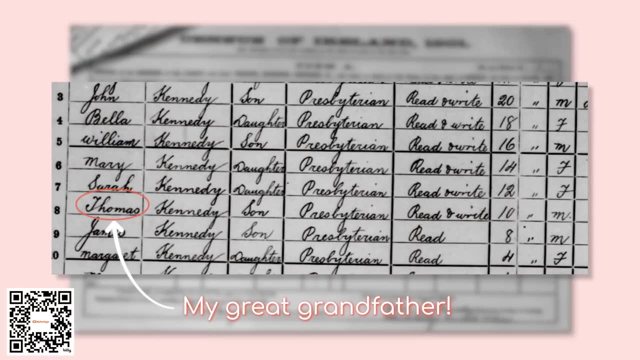 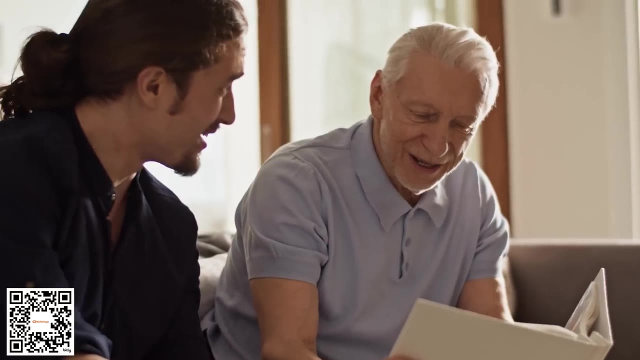 using MyHeritage. MyHeritage's world-leading online service gives you access to over nine 19 million historical records, helping you learn about your ancestors and even discover living relatives you never knew you had. Its AI tools like instant discoveries can help you connect whole branches of your family.